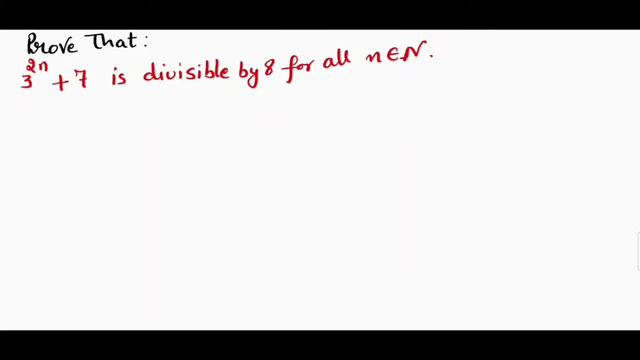 Hello everyone, welcome to my channel. Here we have to prove that 3 raised to the power of 2n plus 7 is divisible by 8 for all natural numbers, And we solve this type of question using principle of mathematical induction. So here, first, what we have to take, we will take Pn, and this Pn is equal to 3 raised to the power of 2n plus 7. 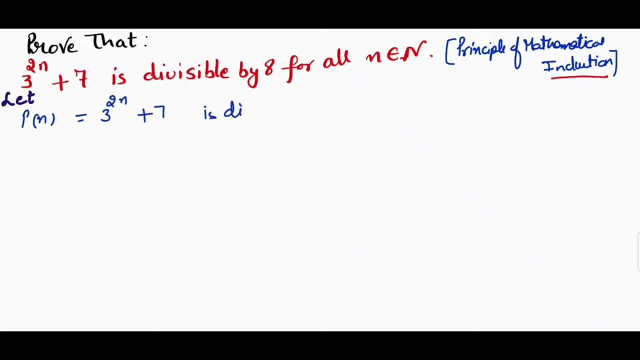 and this is divisible by 8, for all. n belongs to natural numbers. So after that we have to take two steps. Step number 1, we will put n is equal to 1.. So we will see that if we put in this equation n equal to 1, whether this is divisible by 8 or not. 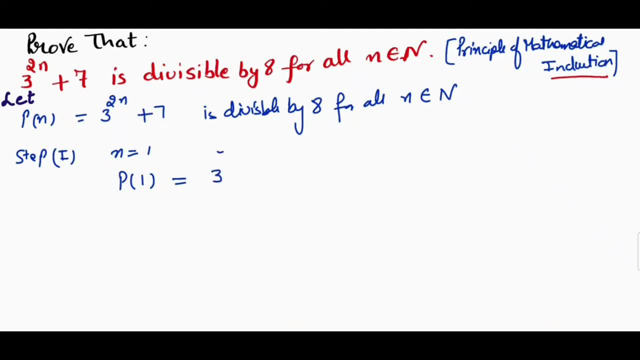 So this will become: P1 is equal to 3, raised to the power of 2n plus 7, which is equal to 3, raised to the power of 2 plus 7, which is equal to 9 plus 7, and this will become equal to 16.. 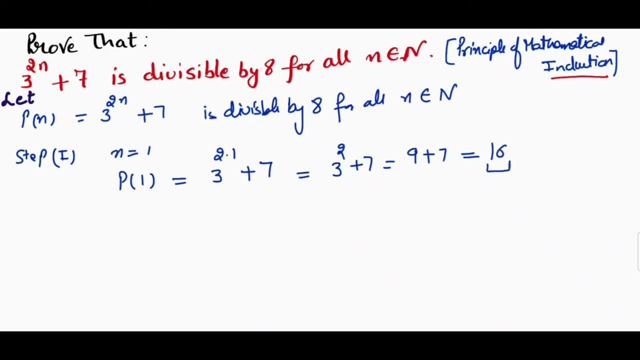 And we know that this 16 is divisible by 8.. So it means P1 is divisible by 8 for all. So next step 2 is here. We will put: n is equal to m And this, if we put this m, then this will become 3 raised to the power of 2n plus 7.. 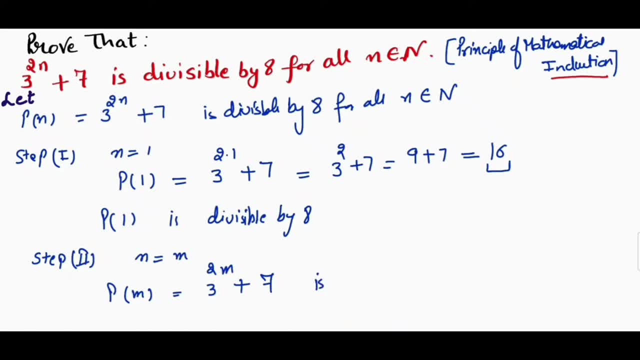 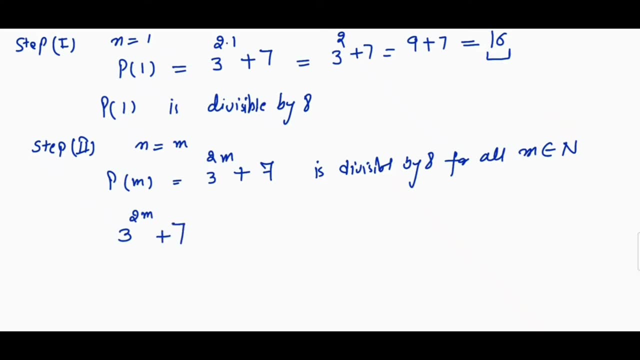 And this is also divisible by 8.. This is divisible by 8, for all m belongs to n. Now I can write this as 3 raised to the power of 2n plus 7.. part 2m plus 7, and it is divisible by 8, is equal to alpha 8. alpha here is any number belongs to. 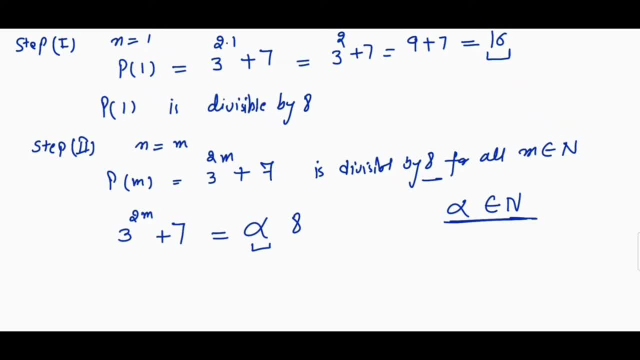 natural number. like this we can write: okay, this will. i'll take this as my equation: 1: now we have to show that p, m plus 1 is also divisible by 8. for that we have to show that. so we have to show that 3, raised to power 2 into m plus 1 plus 7, is also divisible by 8. so for that, 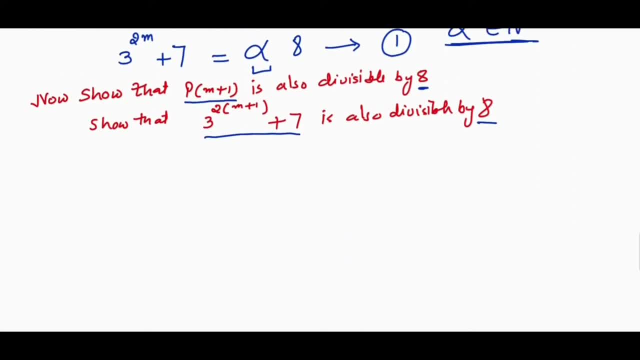 we will do. we can write this as 3 raised to power m plus 1 plus 7. so this we can write like 3 raised to power 2 m plus 2 plus 7. so here i can write this as 3 raised to power 2 m. 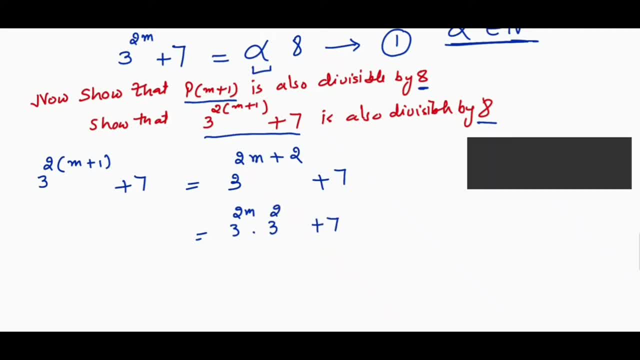 into hospitality to 3 raised to power, 2m plus 7. here I am using this 3 raised to power m into n, which is equal to 3 raised to power m into n. we can write like this: so this will become 9 and 3 raised to power. 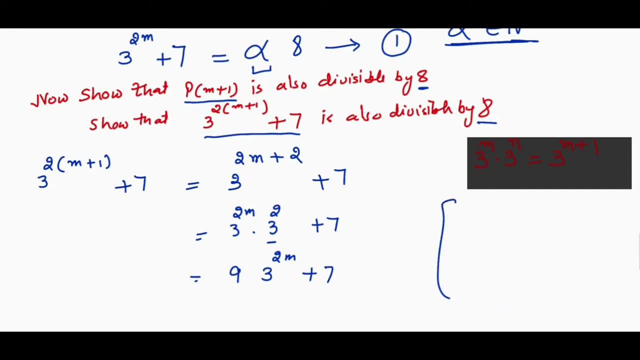 2m plus 7. so from equation 1, see from equation 1- 3 raised to power 2m plus 7 is equal to alpha 8. so from here I can find this value: 3 raised to power 2m will become equal to alpha 8 minus 7. 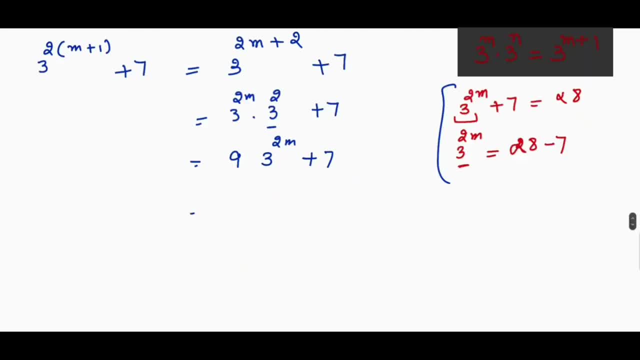 so I will put this value here. so this will become 9 into this alpha, into 8 minus 7 plus 7, so this will become: we will multiply first this, this will become 72 alpha minus 7, and this will become minus. and then 9 and 7, 63 plus 7. so this will become equal to 72 alpha minus 56. so this is. 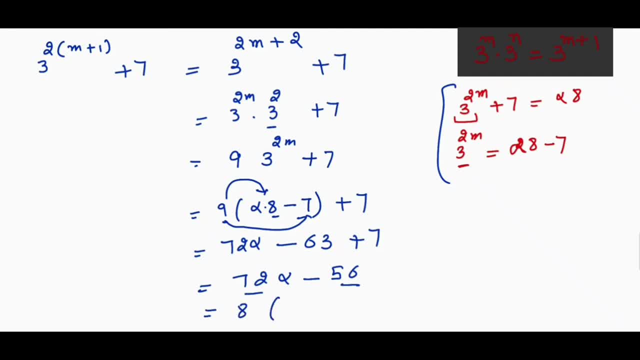 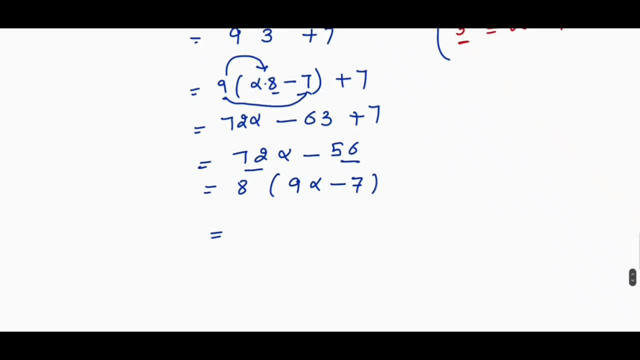 equal to 8 is common. 8 into 9 alpha minus 7, so it means 8 and this whole thing I can take as beta. so this whole thing I can take as beta. so this whole thing I can take as beta, so this whole thing.